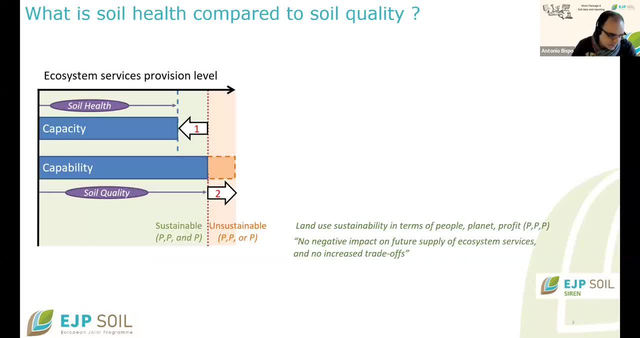 is that, in fact, soil health is not equivalent for us to soil quality, And we developed the following figure to explain the differences between: the difference we think, between soil quality and soil health. And we see, in fact, soil quality as the capability of the soil to support in a sustainable way. 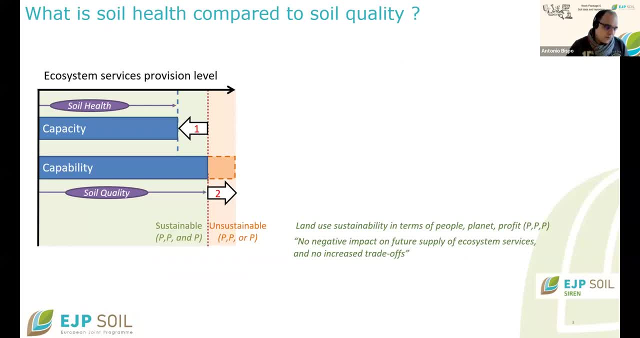 to support the ecosystem services And it's based on the soil properties And then soil health, as just said, is seen as as the current capacity of the soil to support the the ecosystem services, meaning that soil degradation, for example, of non-adapted management practices or climate change. 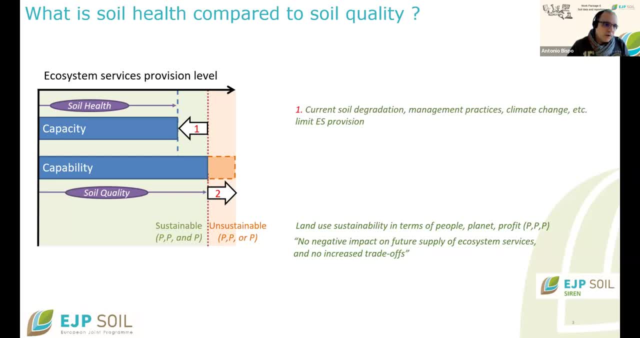 can limit the ecosystem services provision, uh, according to the, to the, to to his capability, in fact. and of course you can also increase the, the capability of the soil, produce more ecosystem services, but then you may have trade-offs on that, so it it may become an unsustainable situation. so that's, that's the way we see the difference between the soil quality. 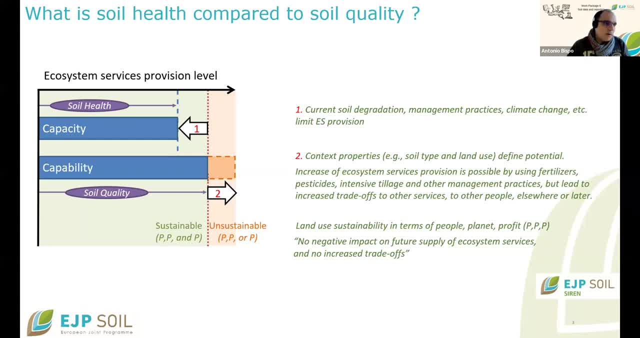 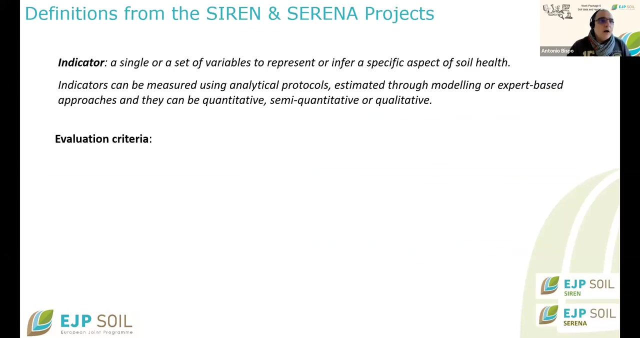 and soil health, meaning that quality is a capability of the soil to sustain, to, to um, to uh, to deliver um ecosystem services, and so the soil health can be seen as a capacity, a current status, a current situation. so there's a difference for us between soil quality and soil health. we also define other 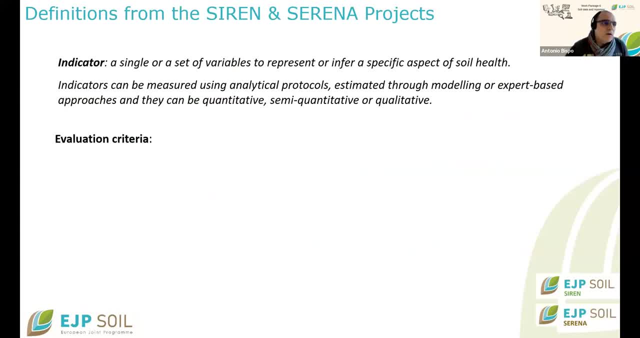 terms like indicator and we see indicator as a single or set of variables to represent or infer a specific aspect of soil health and the indicators can be measured using classical analytical models. and we see that the soil health can be measured using classical analytical models of analysis or different statistical protocols, estimated through modeling or expert based. 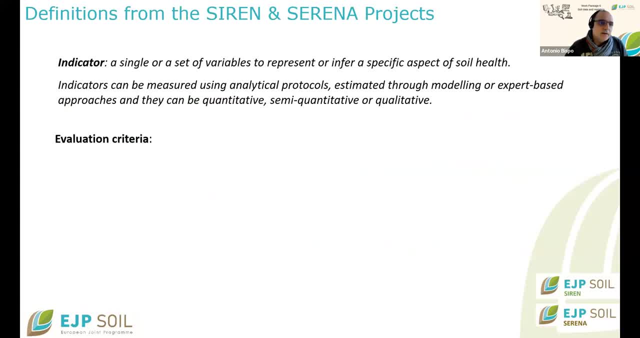 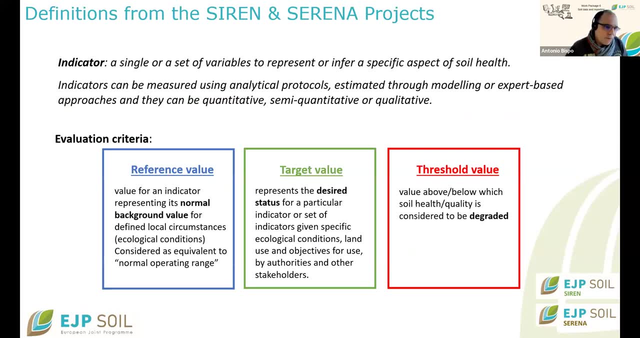 approaches, and then, of course, they can be cantitative, semi-cantitative or qualitative, and we also uh define uh several evaluation criteria as reference value, target value and threshold value. and so a reference value is a value for an indicator representing its normal background value for defined local circumstances. uh, and it's. you can consider it as. 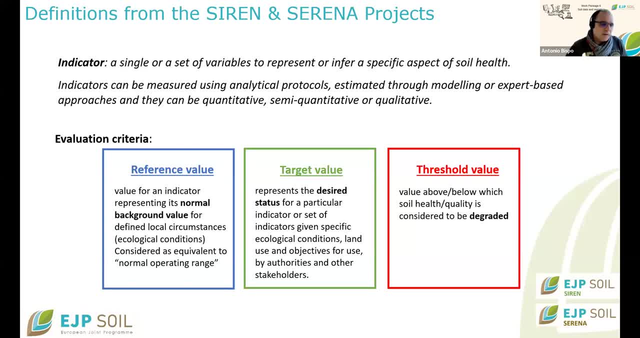 equivalent to normal operating range. that it's. it's also another, another way of saying reference value. target values represent the desired status of a particular indicator or set of indicators giving specific ecological conditions, land use and objectives for use, and it's given usually by authorities or other stakeholders and the threshold is seen as a value above or below which. 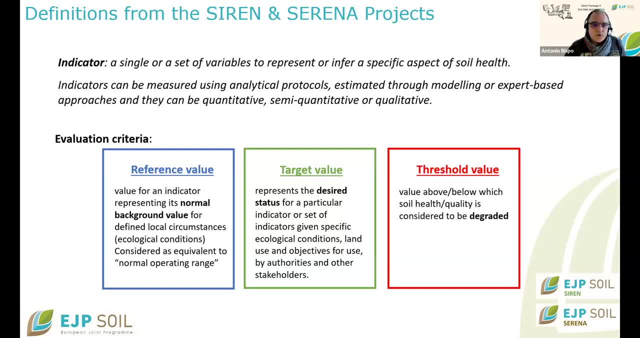 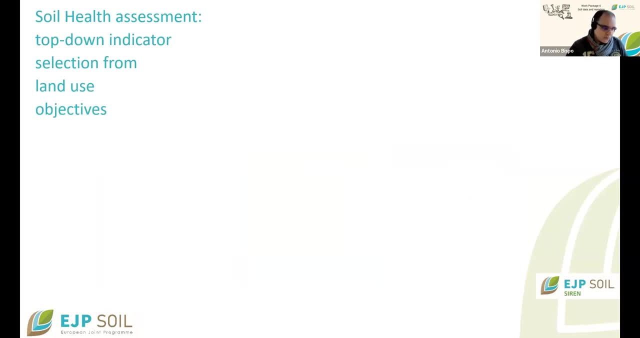 soil health or soil quality is considered to be degraded. so that's, that's the first part on on definitions and then coming to the selection of relevant possible indicators to evaluate soil health or soil quality. we discussed several ways and we first existed a top-down approach and in that top-down, 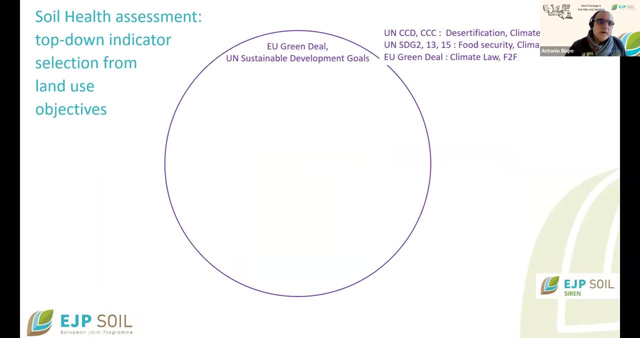 approach. we start from the needs, from the policy needs, and here the there's an example where, if you consider different policy needs for desertification and climate change and food security, then we'll look at what is needed, as what are the ecosystem services that are needed, that are requested to. 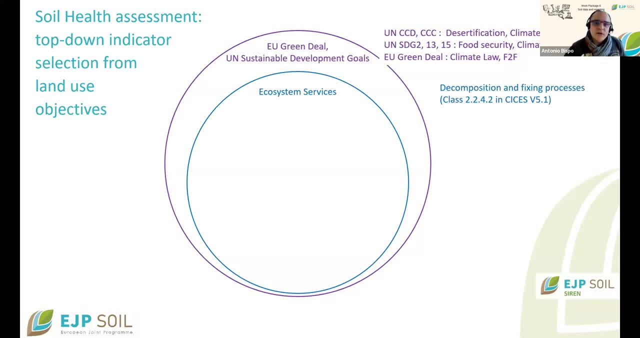 support those policies. then here, for example, it's decomposition and fixing processes linked up to to climate change. and then you look at the, the soil functions that are supporting those ecosystem services. here it's natural soil fertility and balance of soil organic matter mineralization versus humification, and then what are the soil processes behind? 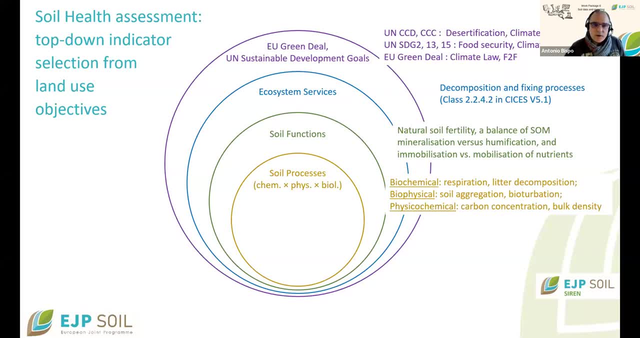 and, based on that, you can choose several indicators: biochemical, biophysical or physical, chemical indicators that will support, in fact, the, the functions, services, and finally, also the, the policies, and again, this is the, the, the, this is uh how we, we define soil quality, integrating those, those different aspects, and we were thinking about that way of selecting uh indicators. 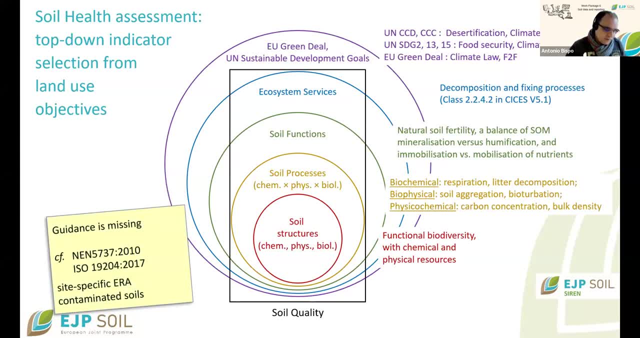 we. we enter the conclusion that the guidance is missing to to to help us to do that. uh, whereas there is a guidance, for example, an ISO document, a guidance to to select indicators for ecological risk assessment, there's a, but there's now a, an ISO working group on on the, on that work that is currently trying to to to. 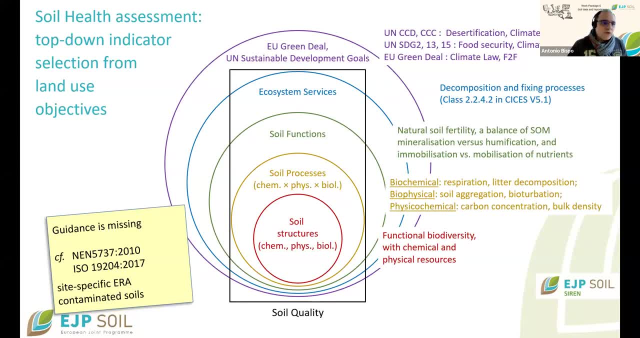 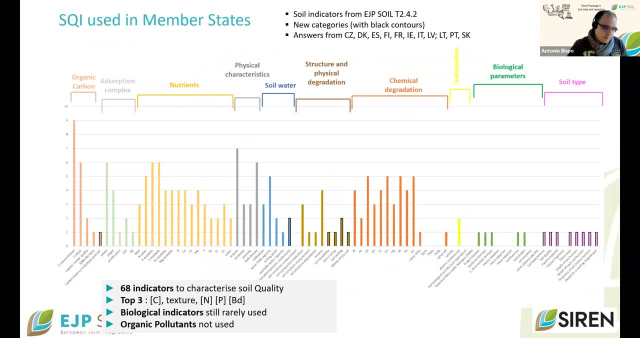 draft that. that guidance uh we also made within uh siren and Serena we we also made a survey within egp solar members to stock take all the quality indicators used in in the countries participating to to to the egp soil program and we got uh several answers uh and those answers are summarized in that figure. 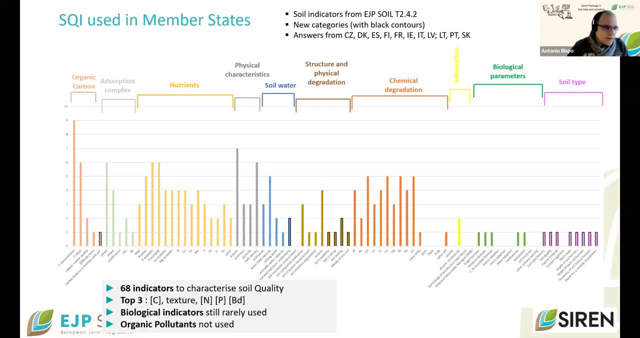 um, we. all the indicators used in the different countries are grouped here by, by categories. you, you see that you have indicators for: for organic carbon, for absorption complex, for nutrients, indicators that report on physical characteristics or on soil, water content, on structural and physical degradation or physical degradation, biological parameters, for example. so, from those 68 indicators, we we then 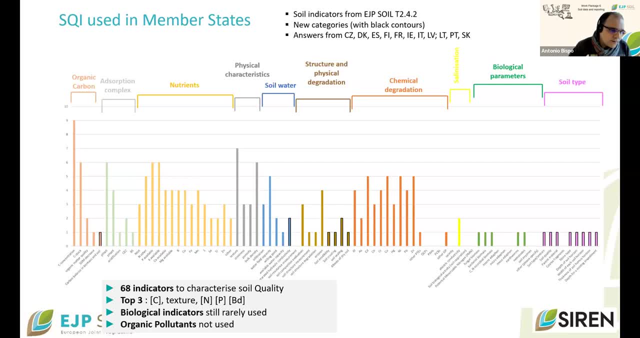 group them and then we identify the top three indicators. so the the the top three indicators are carbon: the measurements uh that report on the carbon status of soils, so it can be carbon concentration, carbon stocks, the organic matter quality- uh, soil organic matter decrease, for example, or carbon balance in biomass and soil. 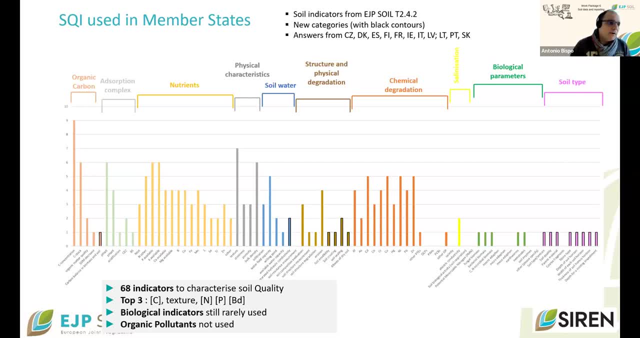 so different kind of indicators reporting on carbon are used in the in the countries, um, uh, you have the number of countries the the y axis is is on the on are the number of countries using the. the indicator and the indicators are are written in in, in in the x-axis, and uh, you can. 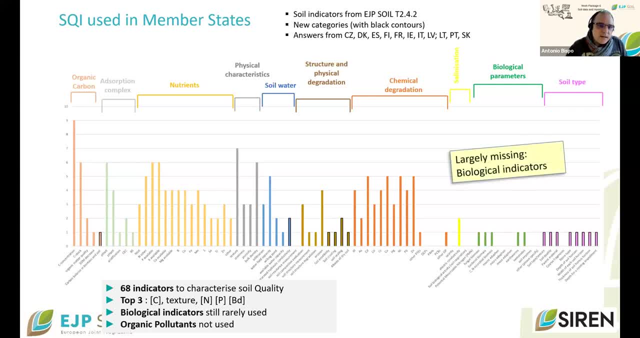 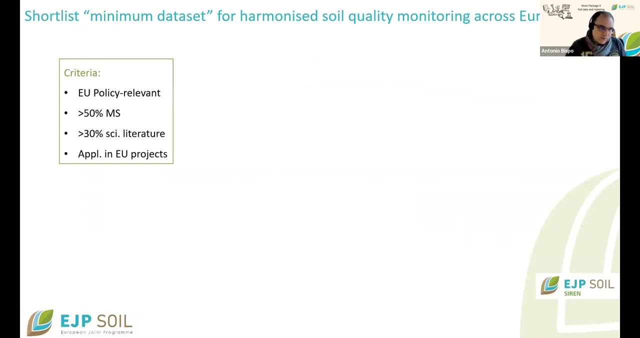 note that biological indicators, for example, are largely missing as a, as in the in the x-axis, so uh, as indicators also on organic contaminants, And so we try to define a minimum data set of indicators for monitoring soil quality across Europe, And so to make that selection. 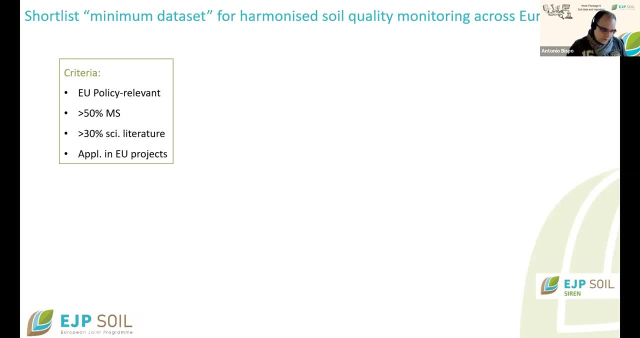 we decide to cross different criteria. And first criteria remember the top-down approach, where those indicators should be policy relevant, They should inform and help policy makers. So first criteria: it should be relevant to policy. Second criteria: it should be used at least by 50% of the countries. 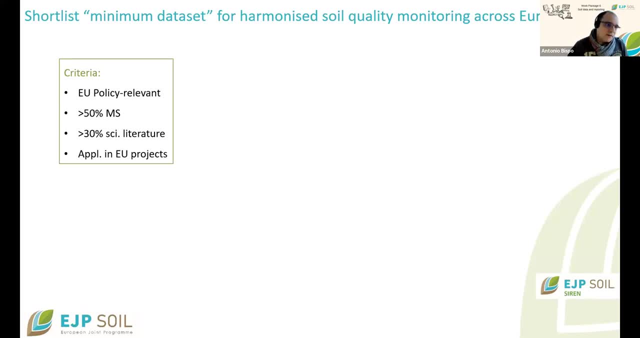 meaning that they are already implemented in several monitoring systems. So we choose that as a second criteria And then the third and fourth criteria where that they should be used in the literature and recommended and also applied and tested in several EU projects. So when you cross all those requirements, 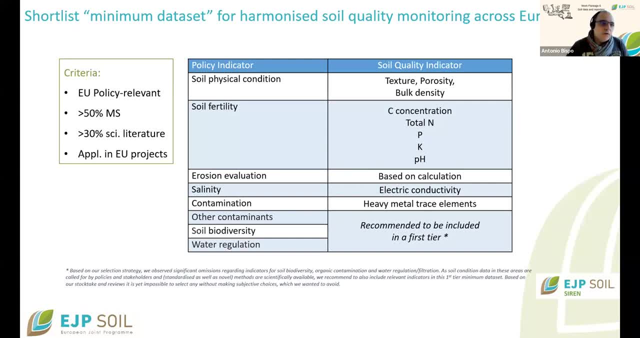 you hand with the following table. So the first column is about the policy relevance of those indicators. They will report on the soil physical conditions, on the soil fertility, on the erosion, on salinity, on contamination, and on soil biodiversity and water regulations. 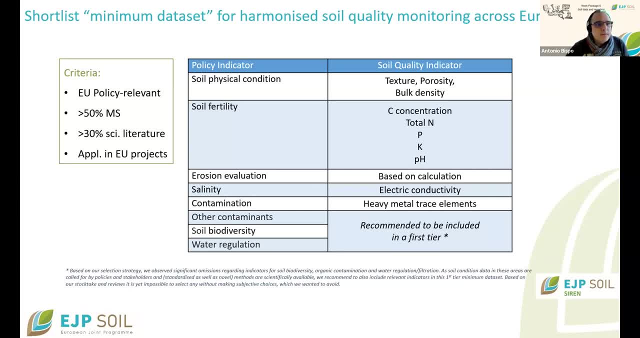 These are the main, the main issues raised by the different policies. And then you have the possible soil quality indicators And you see that for few ones we are missing because they are not used in at least 50% of the countries. The first ones, on texture porosity or carbon concentration. 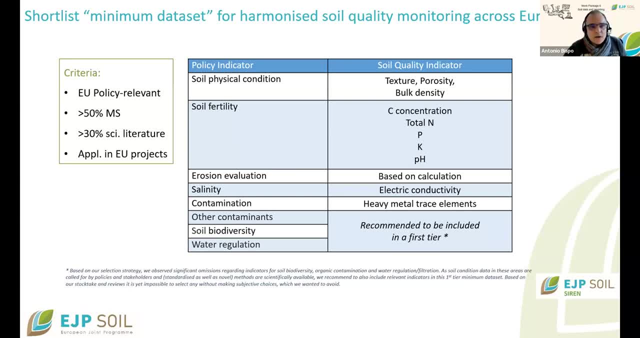 and the gas can already be made using the same told-to1 grader And the other chemistry and terrific data to show, for example, are more snakes 곳inon. but what's a little bit different is that we do not require evidence from the mäjitsä mug Silence. 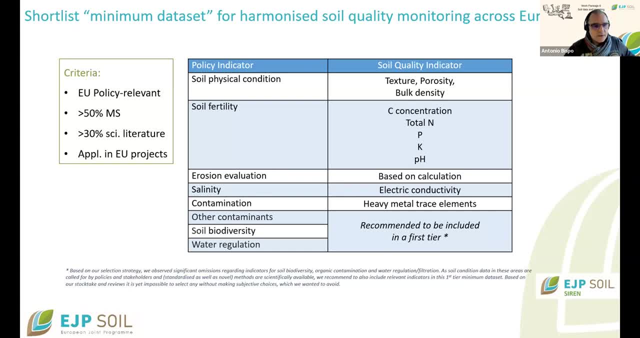 They are already implemented in national systems, whereas organic contaminants, soil, biodiversity and water regulation all notes, And so we recommend to include indicators dealing with organic contamination, soil biodiversity and water regulation. We recommend to include that in a first year, Plus the the other ones that are more or less already used in the countries. 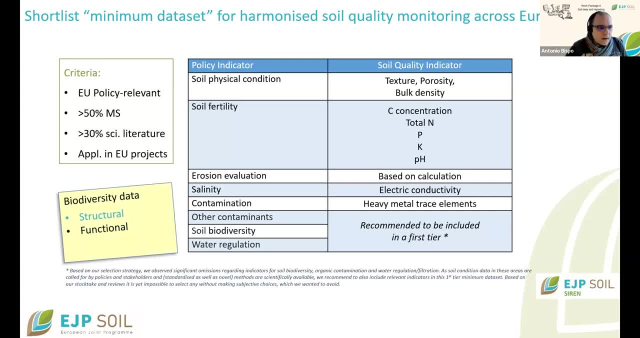 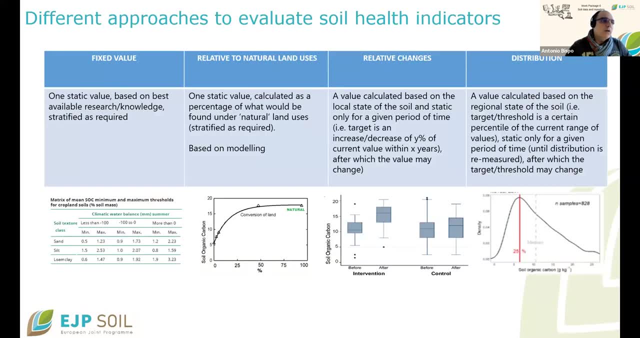 we recommend also to to to collect data on structural and functional biodiversity. so last part of the talk will be on the different ways of interpreting the values, how to set target or threshold values, and so we all together identify four main ways of deriving such values. the first one, quite simple is- is to use a fixed value, one static value based on the. 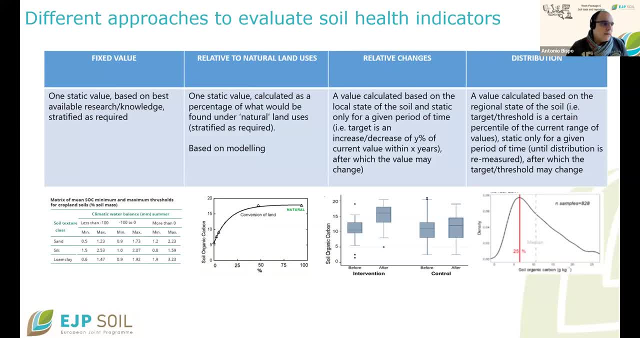 best available research knowledge and, of course, you should also maybe stratify if required and for example, as an example, you have a table that that is proposed by a recent eea report and that developed that proposed values: soil, organic minimum values and maximum threshold for crumple. 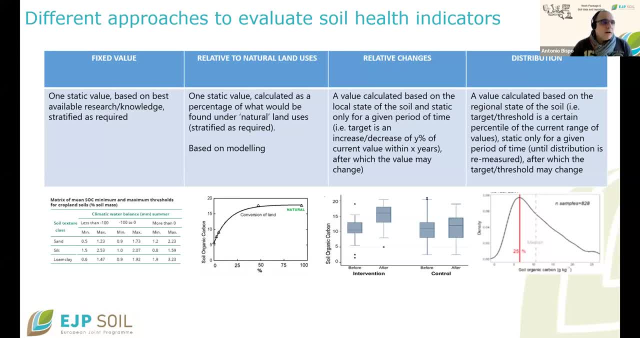 in soils in europe. the second way of providing threshold or target values is to use modeling and and to to to try to have as as an objective a natural situation, a natural land use that could be, for example, like grassland, and then you, you use a model to predict the what could be the situation if, if you change the land. 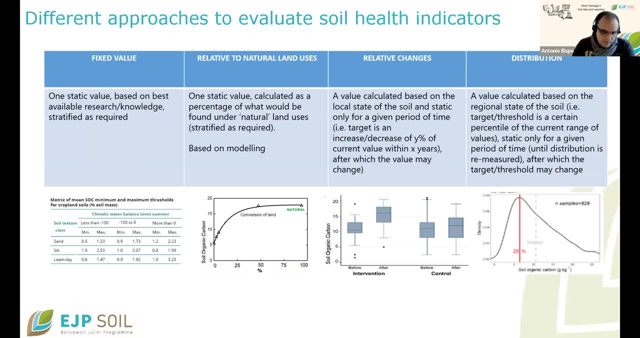 use. if you have a grassland and you set a limit, for example, 60 of that maximum will be your target value and it's based on a modeling approach, the third one in that third one. so you have a graph for that, for that modeling approach. so you, you, you can say that you need to to to reach at least six. 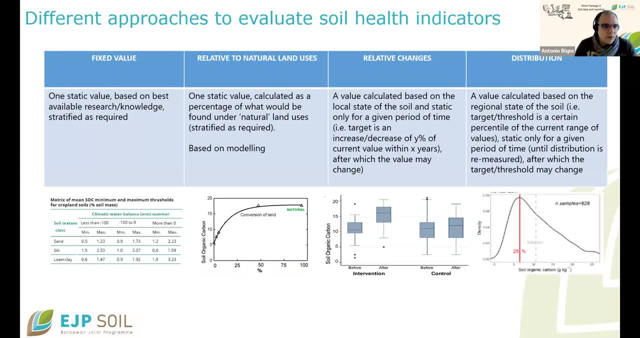 60 percent, for example, of the, of the nature of the natural situation, the. the third way of deriving such values is just to, to give a relative change to, to ask uh for uh an increase or decrease of y percent uh in the coming five or ten years, for example. so you ask people to look at their. 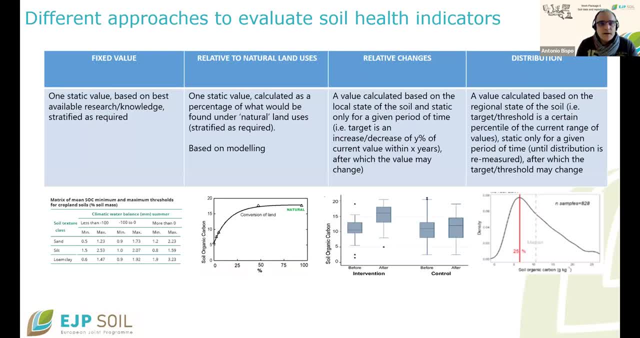 soils and to increase one, one property, one indicator of y percent and to increase y percent on one level, uh, in the coming five years. so it's uh, it's more local, for example, and- and you it can be local or even at national scale- you can ask to increase by five. 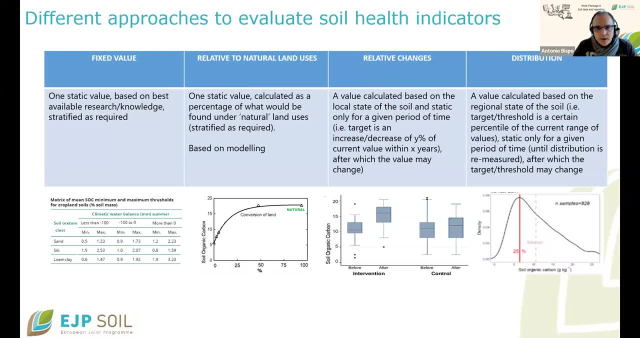 percent, two percent uh, a specific uh parameter of, of of your soils. and the last one is it's a data driven approach, it's based on a distribution. so you, you need for that to um, to make a uh to, uh to, And then you have a distribution of a specific parameter. 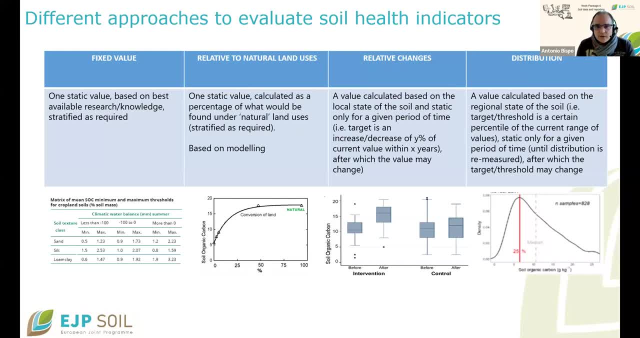 It's, for example, a solar organic carbon, And based on that distribution, you select a certain percentile That will be your threshold or your target value, And this is static, of course. But then if you remeasure it 10 years after, of course the distribution will change. 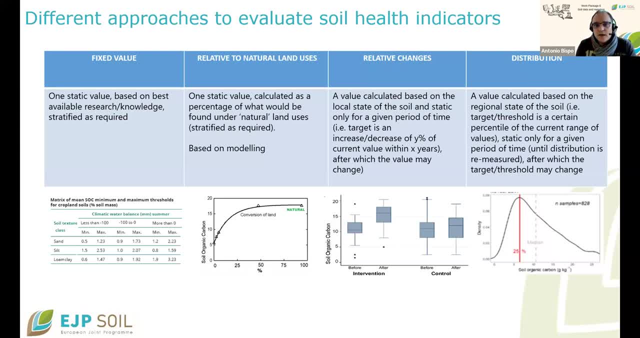 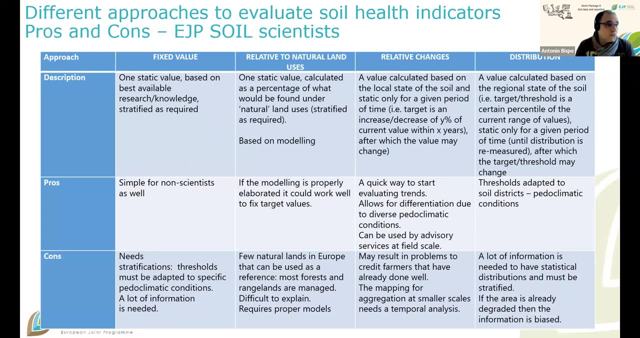 And you can also change your target after that. So you see different ways of developing threshold or target values And we also try to identify advantages and constraints linked to those different ways. And, for example, for the fixed value. well, it's quite a simple way of communication: to communicate the results. 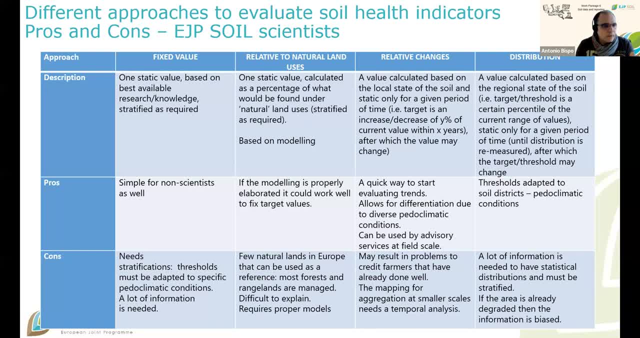 It's easy to understand. You have One threshold- you are about or below, But of course, to do that, you need to stratify according to land use, soil types, for example, And so you need a lot of knowledge for that and a lot of data also. 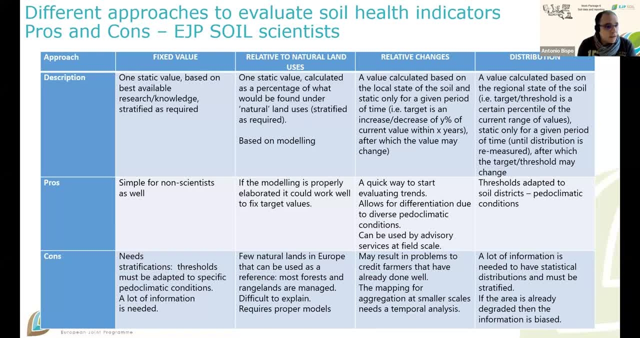 And you also need sort of a consensus between scientists to select the data. The second one, of course. if you have a proper model, it could be quite easily to set those. The second one, of course. if you have a proper model, it could be quite easily to set those. 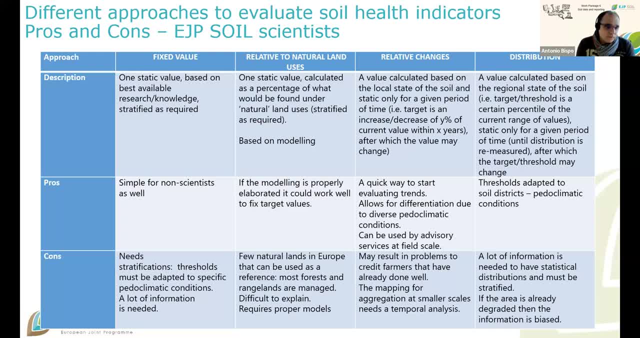 The third one. of course, if you have a proper model it could be quite easily to set those. But then the difficulty is that you need a model, You need a model for different parameters. Then if you set, if the situation is the natural land use, then at least in Europe a lot of landscapes are managed. 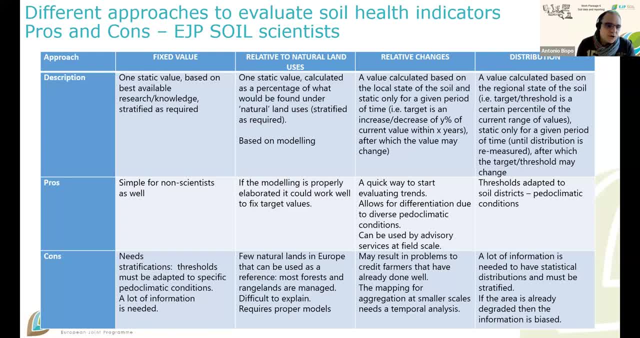 A lot of soils are managed And so there are not that much natural land uses that can be used as a reference, And it's more difficult to explain than a single value. Well, the relative change. it's a quick way to start and look at the trends. 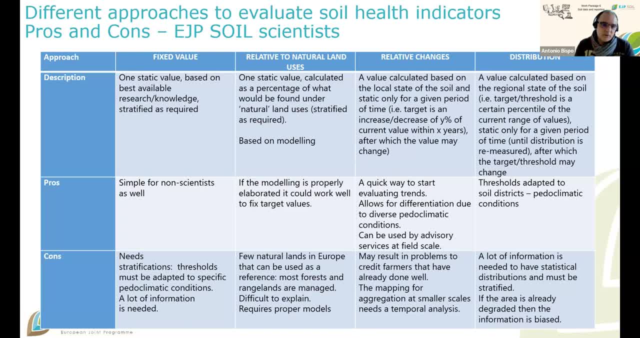 It allows also the differentiation due to diverse pedo-climatic conditions And it can be also used locally for advisory services to help farmers. Of course, one problem is that if you have done very well, if you reach already the target, then it will be difficult for you to improve. 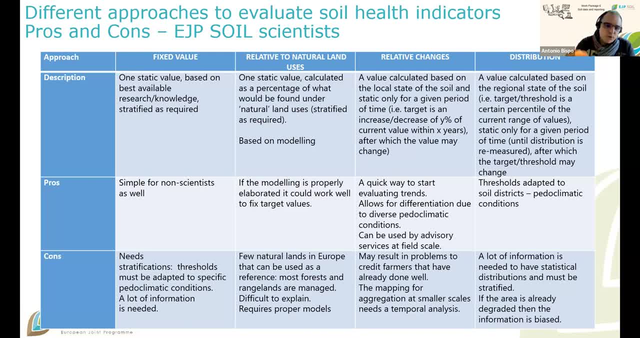 Then if you have done well, it's more difficult to improve then And then you may have also: yeah, if you want to make aggregations and make maps, then you will need to consider also because you have two temporal analysis. you will need to consider that variation in time. 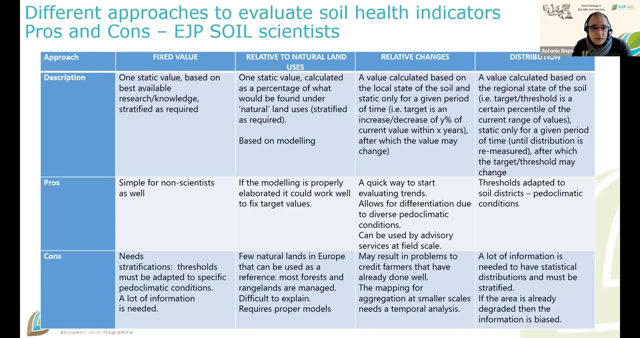 And the last one for distribution. well, it's quite adapted to pedo-climatic conditions, because you can stratify your data according to different districts, according to land use, soil type and climate, for example. But of course, to do that you need a lot of information, a lot of data, to develop those statistical distributions. 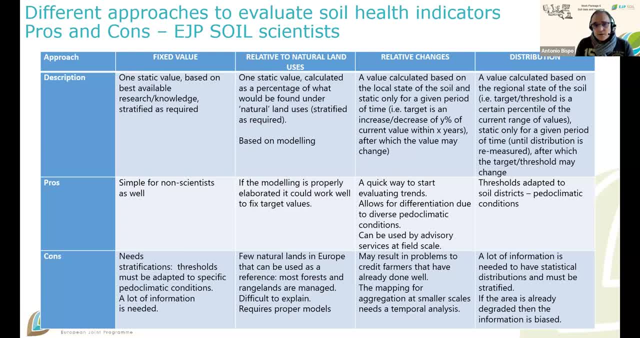 And another point is that the area is already degraded. Then your information is biased, Because your distribution will be pushed to low values, for example, and then the target you are setting is already a degraded situation. It's not, let's say, a normal or a median situation. 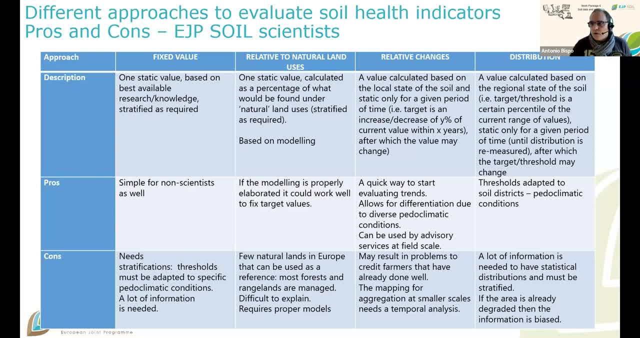 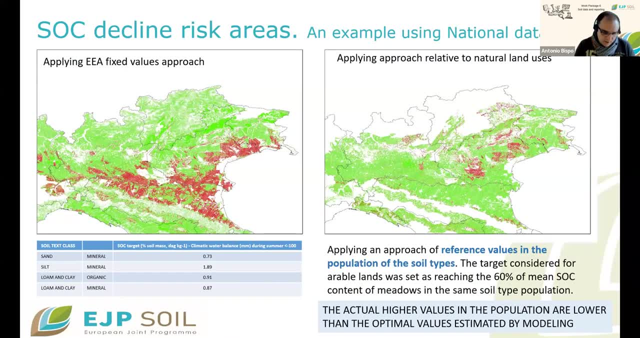 It will be a degraded situation. So we need to take care of that And the colleagues from Italy already tested, are starting to test those different ways of deriving. methods of deriving- Sorry- The thresholds and target values. And so on the left part of your screen you have the. they apply the EEA threshold values. 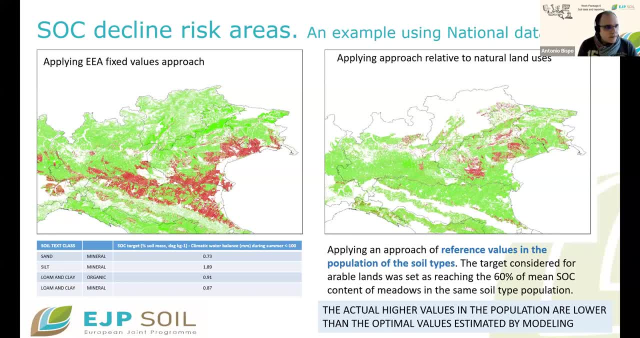 So the table I show you at the beginning, that are stratified according to soil texture, And so you see in red the degraded areas. And if on the right side of your screen they use a reference, they use a reference to natural land use, to grasslands. 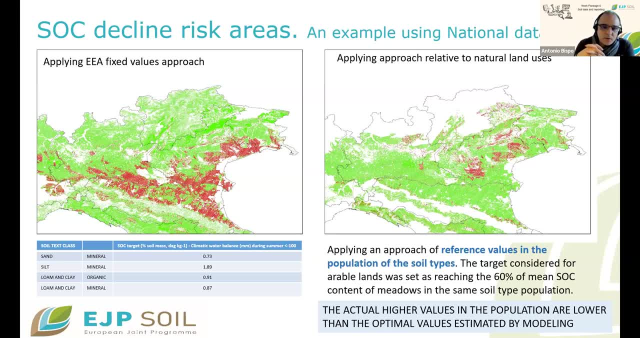 And they set a threshold at 60% of the mean of soil organic content in mediums And you see the difference: You have less red colored areas. So you that means that depending on the choice of your, of your method to derive or target or threshold values, you may end with very different situations in your country. 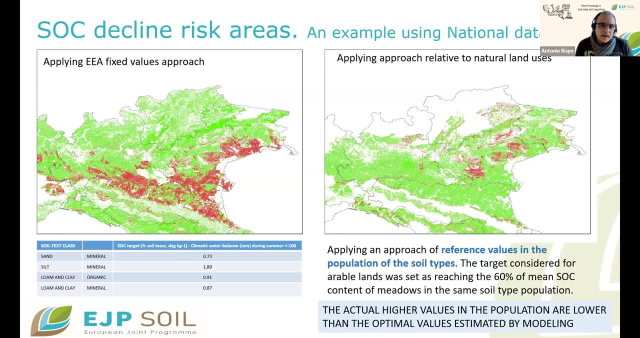 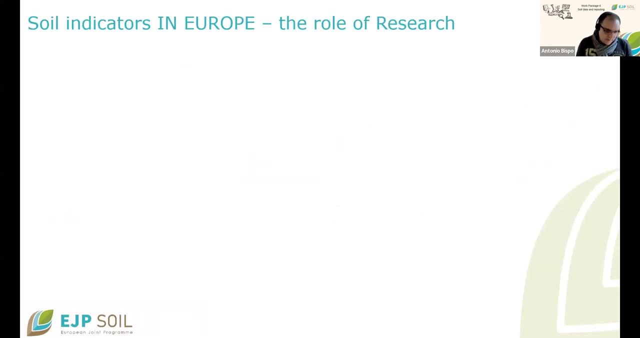 So, yeah, we, we need To to think about that and and and think about how to derive those, those target or threshold values. And finally, I will end with, I try to to set the scene, the current scene of the of this issue of selecting indicators and providing targets and threshold values. 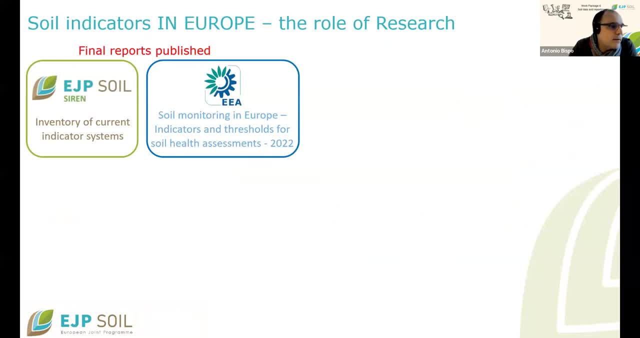 And just to let you know that we talk about the SIREN project that is currently finished and we have the the the report available and also the EEA report on soil monitoring in Europe and that that also propose indicators and thresholds for soil health assessments. 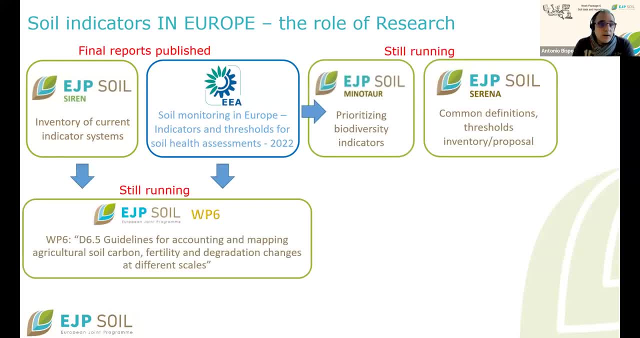 So these documents are available. Still running the the EGP soil projects Minotaur and Serena. You will have a presentation just after of of those projects, Thank you. And still running also the work package six of EGP that and we deal with the development of indicators and thresholds and we are currently drafting a, a guideline for that. 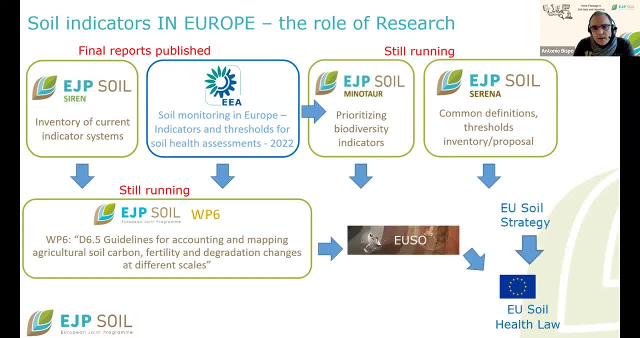 And everything is now is feeding the: the European soil strategy, the European soil law and the European soil observatory. And remember that, just starting now, two other projects from the EU mission that are starting a benchmark, and all four Soil, So two projects that will also update our vision on indicators and the thresholds or target values. 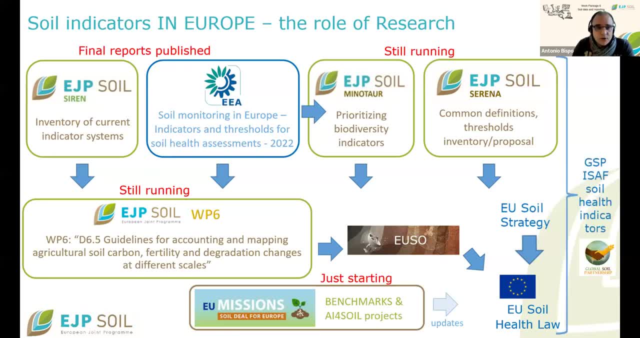 And finally, everything, every reflection should also help the building of a, of a new indicator that is now proposed by the global soil partnership on soil indicator. So the story is not finished. There is a huge place now still for for research.